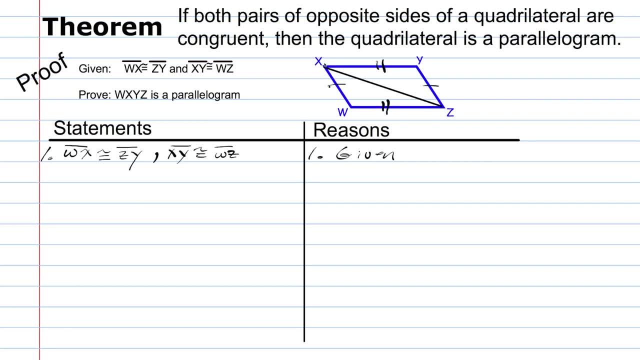 parallel to side WZ, Then we have to prove that side XW is parallel to side YZ. To prove lines parallel we have to focus in on the special angles formed by parallel lines. in a transversal That would be: alternate interior angles, alternate exterior angles, same side interior angles. 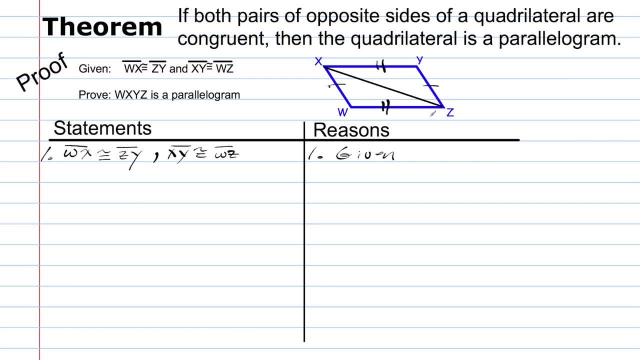 or supplementary Things like that, And a lot of times the proofs for parallelograms have to do with alternate interior angles. For example, if we take a look at side XY and side WZ as our parallel lines and we'll mark those with this red dash line, just to give you an idea. 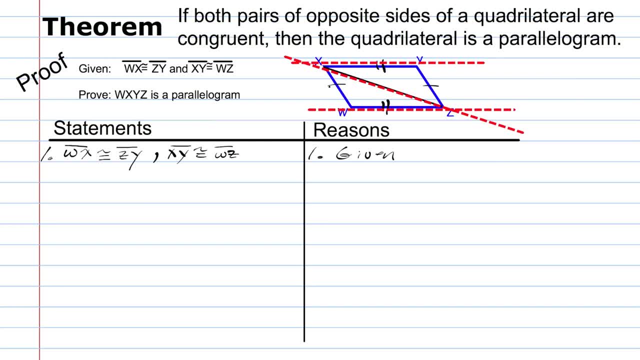 And this is our transversal Alternate interior angles, in this case would be: right here, Which I'm going to label angle 1.. And right here, which I'm going to label angle 2.. So to prove that line XY is parallel to line WZ, I need to prove that angle 1 and angle. 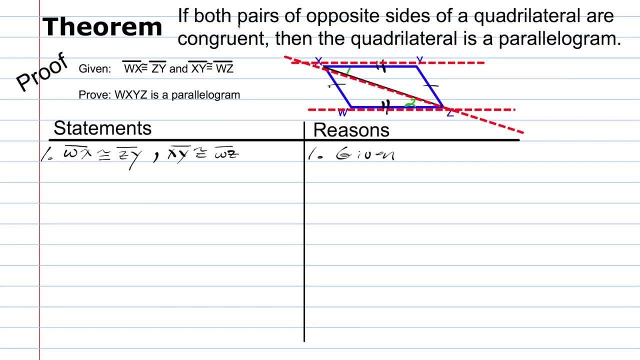 2 are congruent On the other side of that, if I look at side WZ being parallel, or what we hope to be parallel lines crossed by a transversal, transversal, and WZ- the angles that we're going to need to prove congruent to one another. 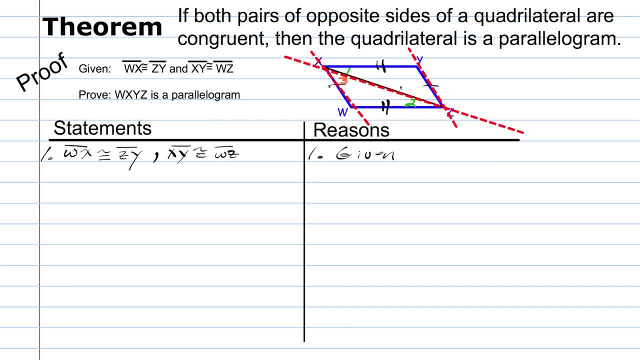 are the alternate interior angles here, which would be right, here, which I'm going to label angle 3, and here, which I'm going to label angle 4.. So we need to prove those two angles congruent to each other, to prove that these sides are. 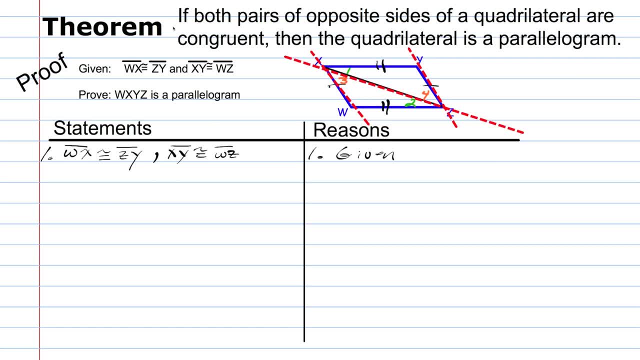 parallel. Well, to prove that they're congruent, we're first going to have to do a triangle proof. So let me get rid of these red lines And now we can start our proof, because ultimately, what we have to do is prove angle 1 congruent. 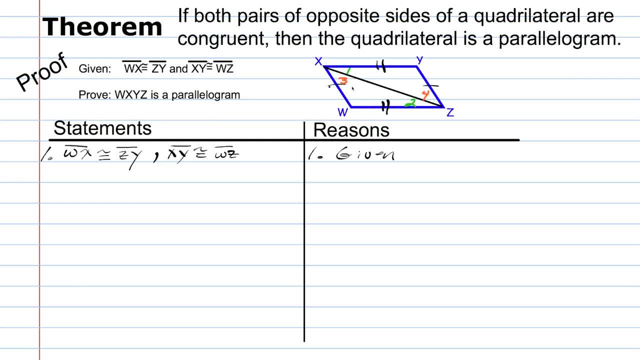 to angle 2, and angle 4 congruent to angle 3.. And to do that, we're going to prove this triangle on the bottom, triangle WXZ, and then triangle ZYX, congruent to angle 3.. So the first step to proving these two triangles congruent is going to be to prove that XZ is. 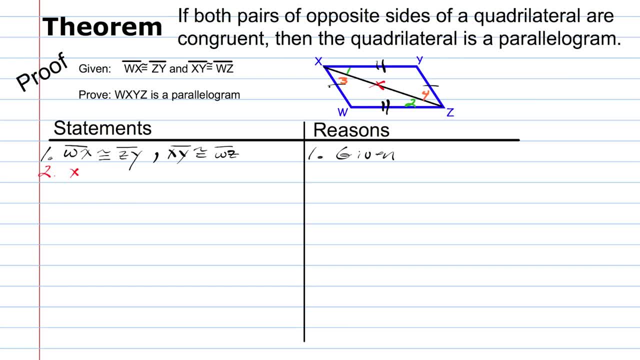 congruent to itself by the reflexive property. Segment XZ- not XY, but XZ- is congruent to segment XZ and that's because of the reflexive property of congruence. Now that we have, and if we look at the top and bottom triangles, if you will, we have- 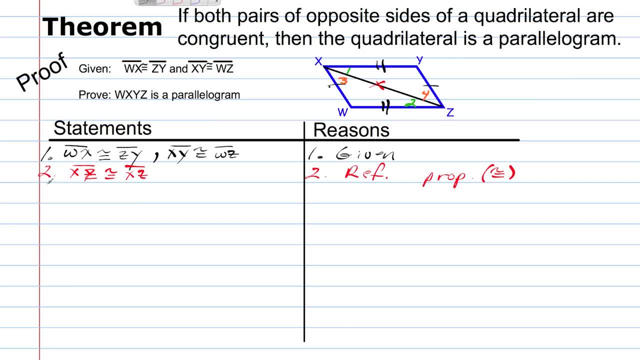 side side side. So we can make this statement: the triangle XYZ is congruent to triangle ZWX And that's why these sides are congruent. Okay, All right, Let's do that. Side side side postulant. 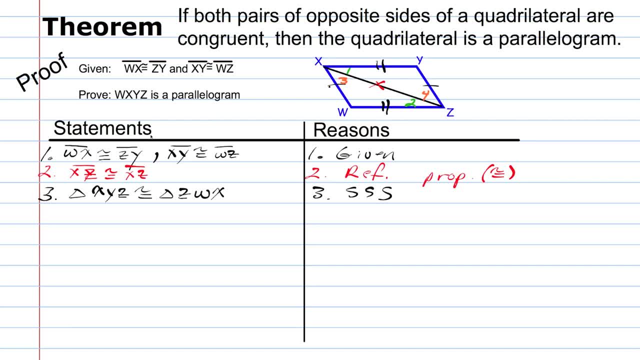 Triangle congruence- Side side side. Now that we have the two triangles proved congruent, we can prove that the angles- angle 1 and 2, and then angles 3 and 4- are congruent. We'll do that in red. 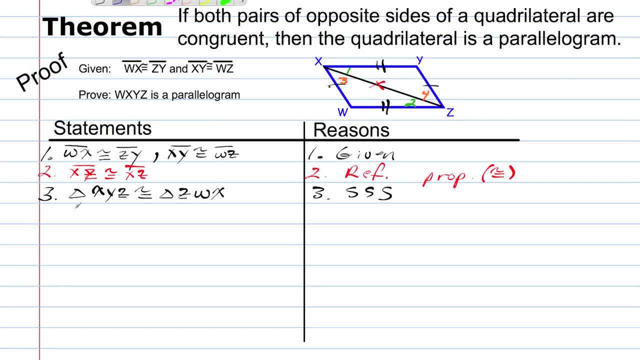 Actually we're going to do that in blue. So the fourth step is going to be to say that these are congruent. So angle 1., 2., 3., 5., 6., 7., 8., 9.. 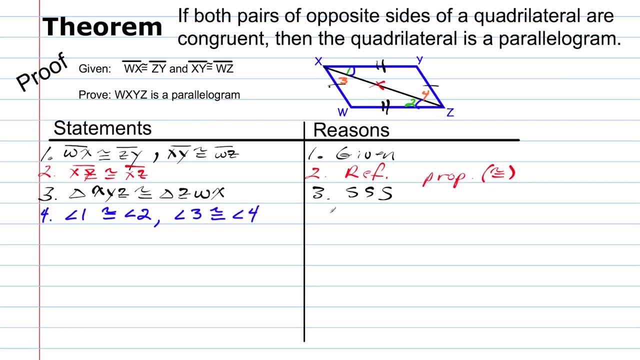 10., 11., 12., 12., 13., 14., 14., 15., 16., 17., 18., 19., 20., 21., 22., 23., 24.. 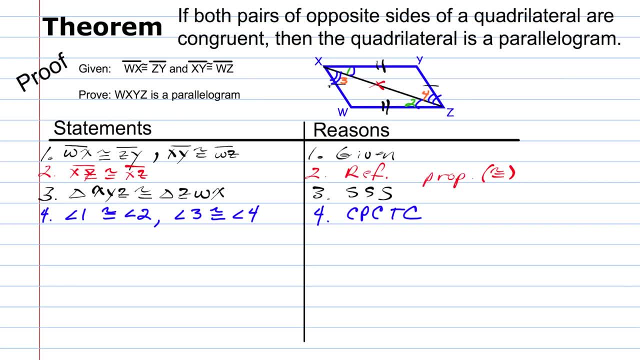 25., 26., 27., 28., 29., 29.. is that the opposite sides are parallel to one another. We can say that xy is parallel to wz. So segment xy is parallel to segment wz. And remember that's because angle 1 and angle 2. 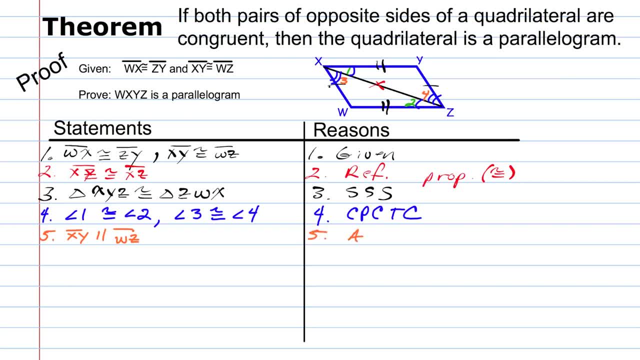 are congruent. The reason for that is the alternate interior angles theorem. The alternate interior angles are congruent, then the two lines are parallel. The other statement we can make is: xw is parallel to yz And again that's for the same reason: the alternate interior. 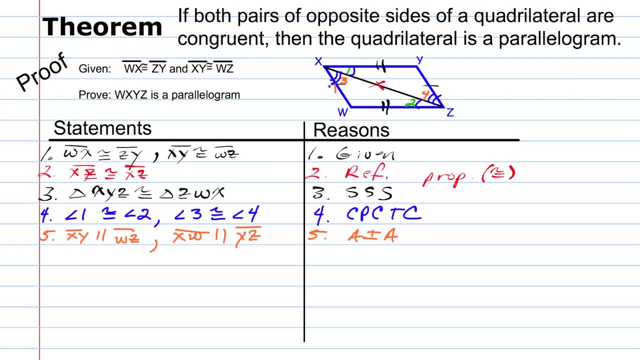 angles theorem. So we have the opposite sides now marked parallel, not congruent. That's what these arrows mean: that they are parallel. And since we have opposite sides parallel, we can state that the quadrilateral is a parallelogram. So in this case, wxyz is a parallelogram. 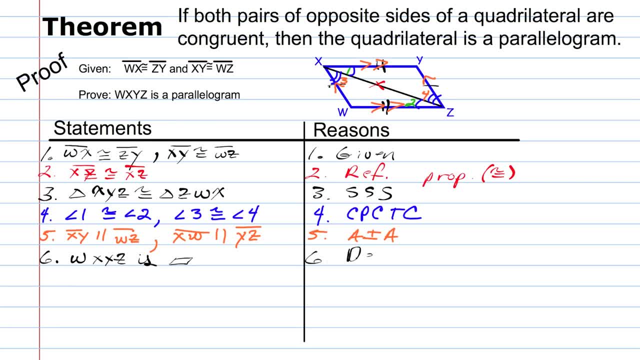 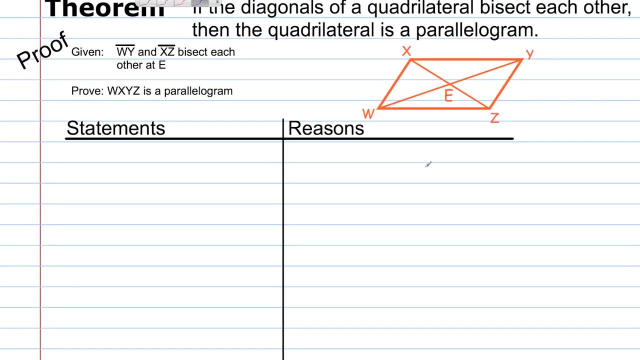 And that's because of the definition of parallelogram. Again to review. I proved the two triangles were congruent so that I could prove the angles Which were alternate interior angles were congruent, to prove the sides parallel. This second theorem that I'm going 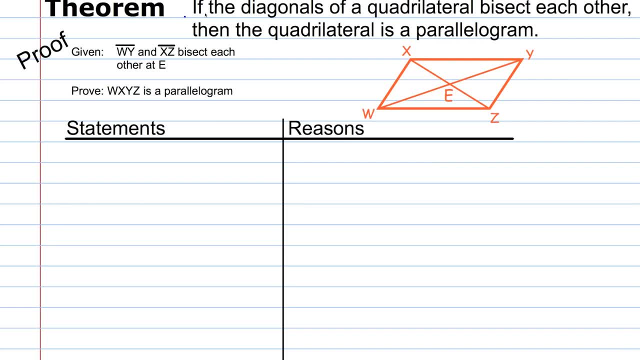 to write a proof for today reads: if the diagonals of a quadrilateral bisect each other, then the quadrilateral is a parallelogram. Again, a parallelogram proof or proving a quadrilateral is a parallelogram In this case, since we're told that if the diagonals of a quadrilateral bisect each other. 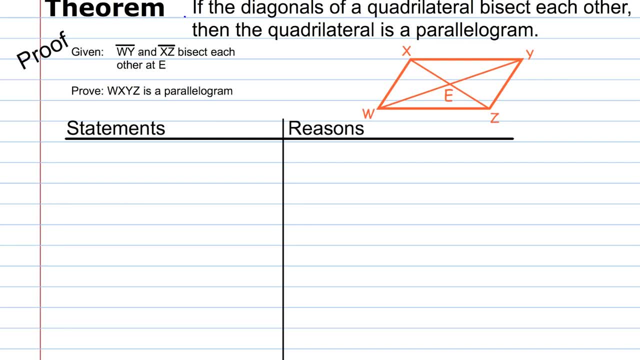 then the quadrilateral is a parallelogram In this case, since we're told that if the diagonals of a quadrilateral bisect each other, our given matches that. It tells us that the diagonals diagonal wy and xz bisect each other at e. 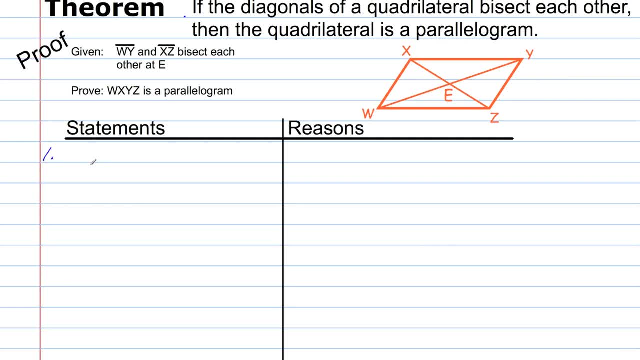 So we can go ahead and write that into our given Segment: wy and xz bisect each other at e. So that's our given. Now, that's our given, Much like the last proof. parallelogram proofs are really going to be dealing with proving. 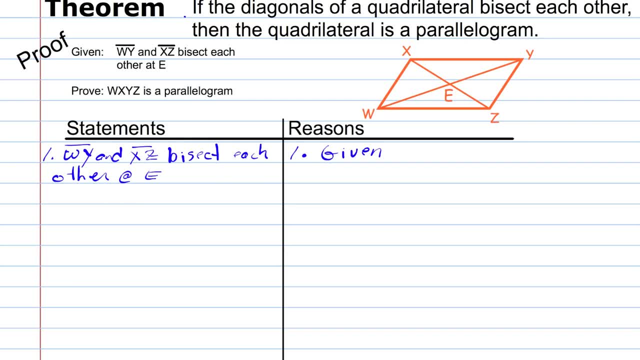 the opposite sides or parallel, by using alternate interior angles theorem. So to identify here, if we take a look at sides wx and zy, That's one pair of sides that we need to prove parallel. Alternate interior angle would be here And here what I'm going to label angle 1 and angle 2.. 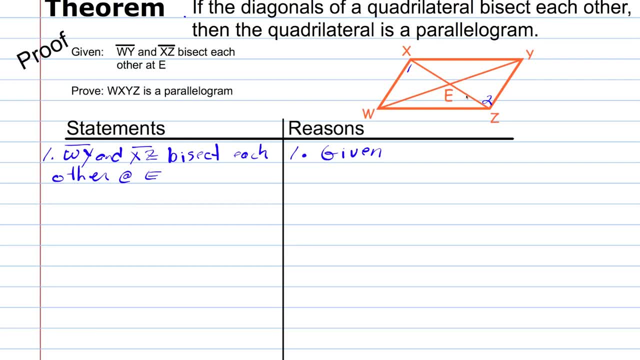 If we can prove those two angles are congruent, then WX and ZY would be parallel. If we take a look at the other sides, the other pair of opposite sides, XY and WZ, the alternate interior angles we're going to be working with are going to be here and here 3 and 4.. 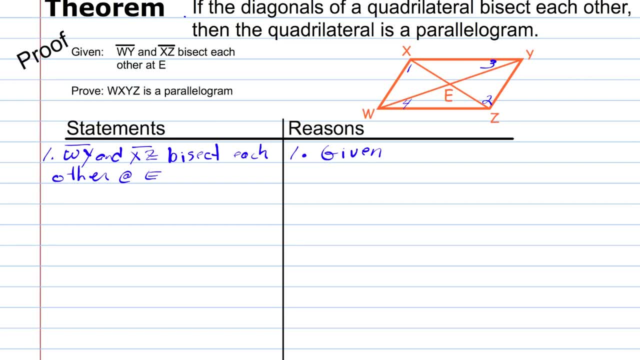 If we can prove those congruent, then segment XY is going to be parallel to segment WZ by the alternate interior angles theorem. To prove them congruent we're going to use a triangle congruence proof. So let's get proving angle 1 and angle 2 congruent, angle 3 and angle 4 congruent. 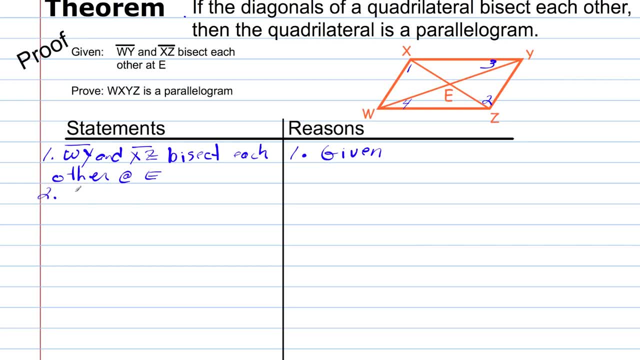 The second step of our proof is to actually say that XE or segment XE, is congruent to segment ZE. we'll mark those congruent now, and the other part of that is that segment WE is congruent to segment YE. 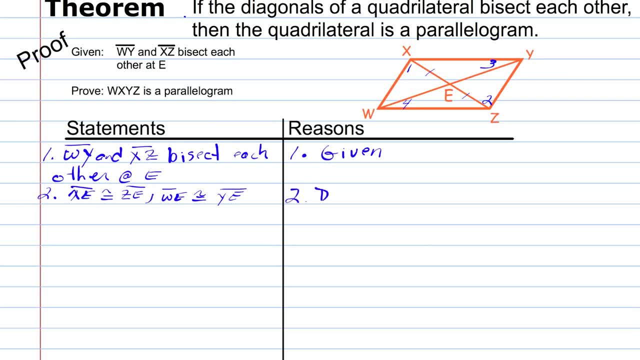 And that's because of the definition of segment bisector, So we can mark these two congruent to each other. The third step is to mark the vertical angles congruent, And in here we can say that angle XEY is congruent to angle ZE. 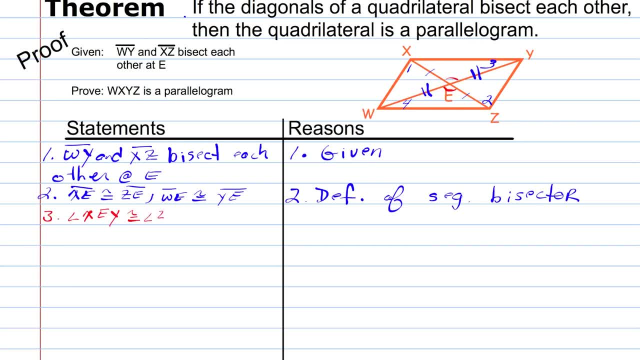 And we can also say that angle XEW is congruent to angle ZEY, And that's because of the vertical angles theorem. Now, what we have is that we have this top triangle triangle XEY and this bottom triangle, angle ZEW congruent to one another. 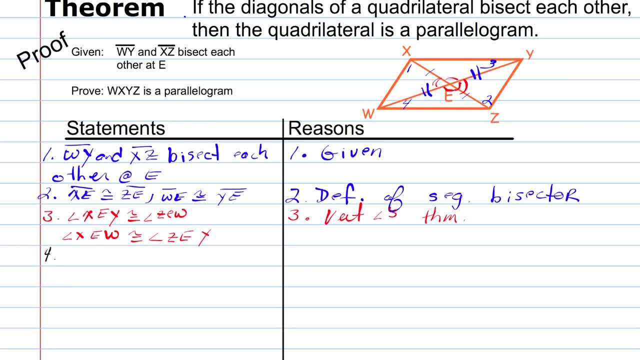 And that's because of side angle side. then we also have the left and the right triangles. So triangle XEY is congruent to angle ZEW And that's because of the vertical angles theorem. So triangle XEY is congruent to angle ZEW. 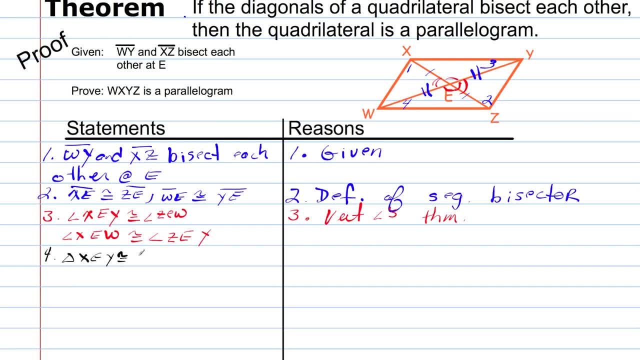 And that's because of the vertical angles theorem And that's because of the vertical angles theorem. It's congruent to triangle ZEW and triangle XEW. It's congruent to triangle ZEY And the reason for that is the side angle side. 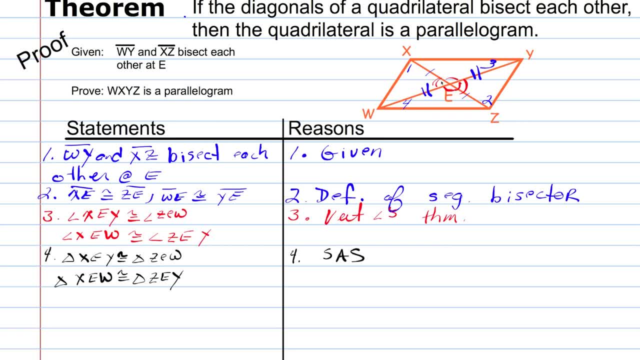 Again, it's the top triangle congruent to the bottom triangle and the left triangle congruent to the right triangle. Now that we have that established, what we can do is we can now establish that angle 1 is congruent to angle 2, because angle 1 corresponds to angle 2 in the left and the 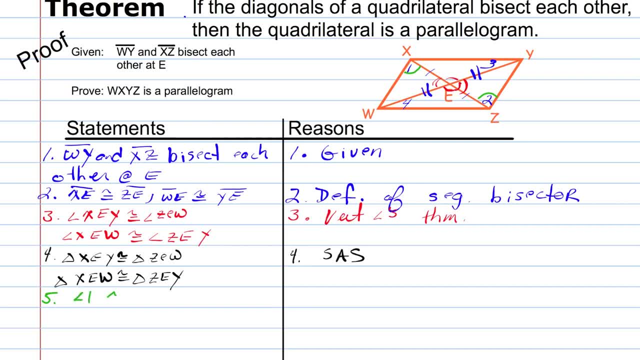 right triangle. So we'll be able to say that angle 1 is congruent to angle 2, and, for the same reasons, angle 4 is congruent to angle 3, and that's because the corresponding parts of congruent triangles are congruent. 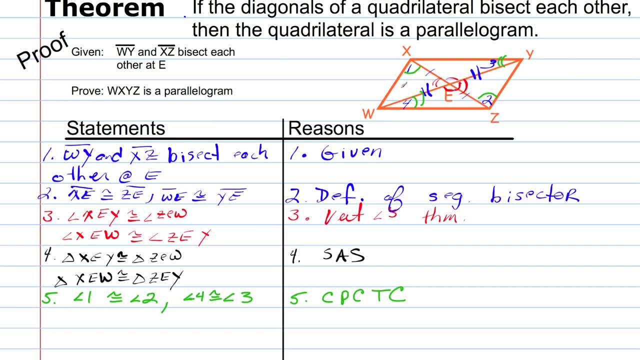 Now here's the cool part. Angle 1 and angle 2 are the alternate interior angles to side W X and Z Y. so now we can say that those sides are parallel. We can say that W X is parallel to Z Y. I'm going to mark that with a single orange. 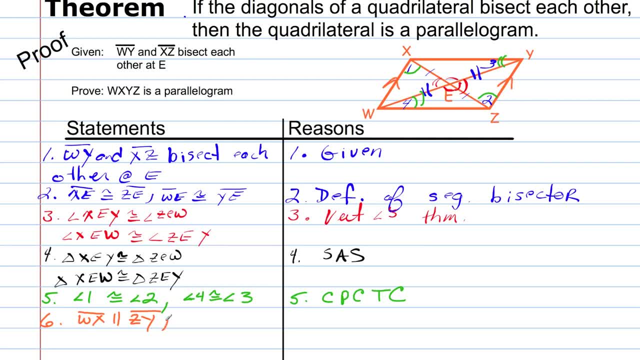 arrow, meaning that these two are parallel. and we can also say that the top and bottom lines are parallel because angle 3 and angle 4 are congruent to each other, which are alternate interior angles. So angle X, Y is parallel to side W, Z, and the reason those are parallel is because of the alternate. 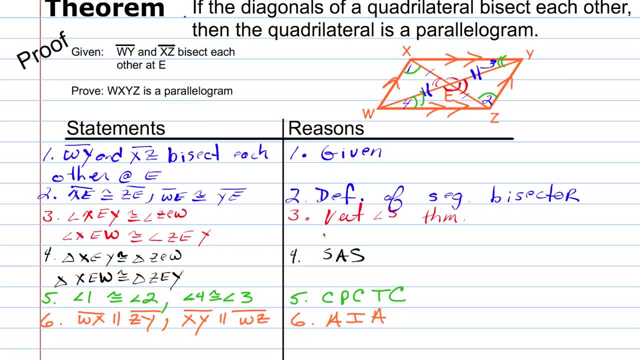 interior angles theorem. Now, finally, now that we have opposite sides of this quadrilateral parallel, we know by definition that the quadrilateral W X Y Z, X Y Z, X Y Z is a parallelogram, and that's because of the definition of parallelogram. 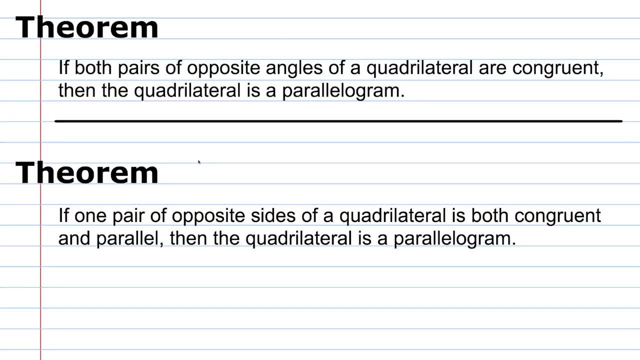 Here we have two more theorems in this video geometry lesson that we're not necessarily going to prove in the video. These will be left for my students to complete as exercises in or outside of class. The first theorem here is: If two pairs of opposite sides of the quadrilateral parallel are congruent to each other, then 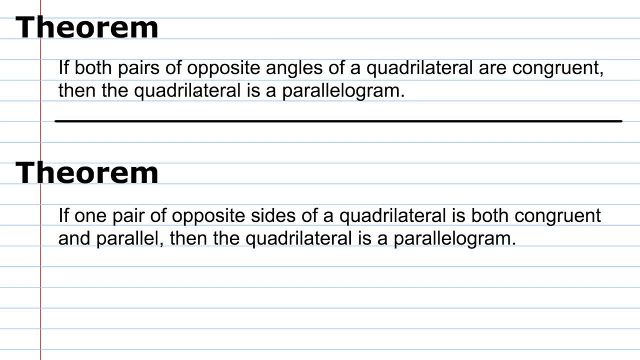 we're going to have two pairs of opposite sides of the quadrilateral parallel. If two pairs of opposite angles of a quadrilateral are congruent, then the quadrilateral is a parallelogram. So if we can establish that the opposite angles are congruent, then we can conclude that the 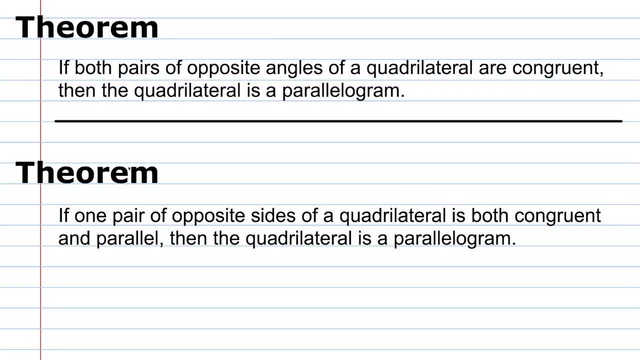 quadrilateral is a parallelogram. The next theorem here is: If one pair of opposite sides of a quadrilateral is both congruent and parallel, then the quadrilateral is a parallelogram. So here, If we can identify that just one pair, 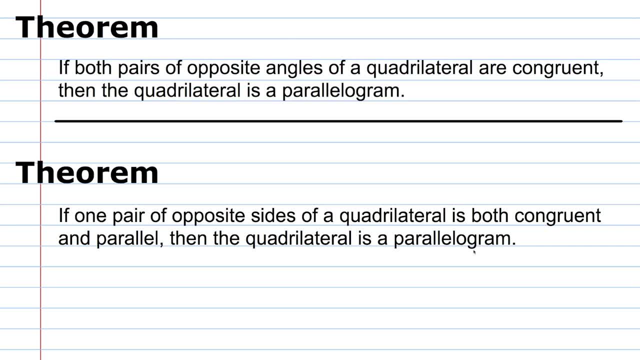 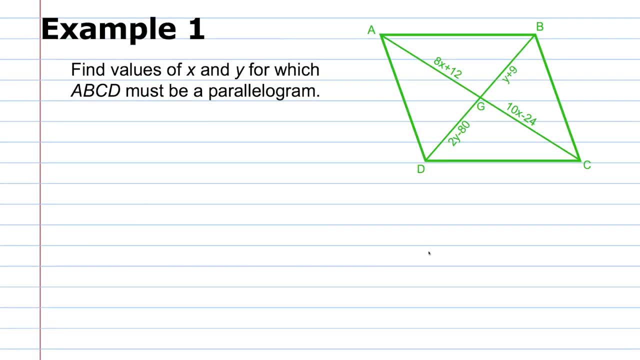 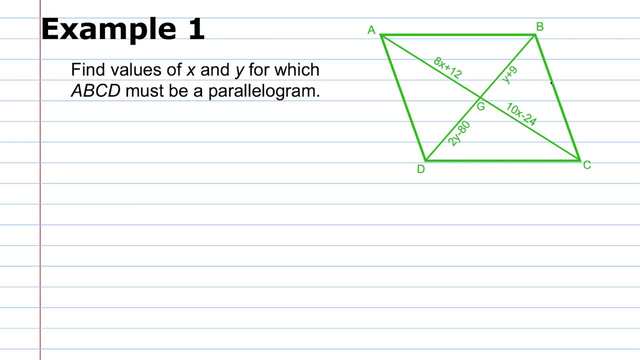 X, X, X X X. We are given information about the diagonals and for this shape to be a parallelogram, the diagonals bisect each other, which means that this right here, 8x plus 12, must be. 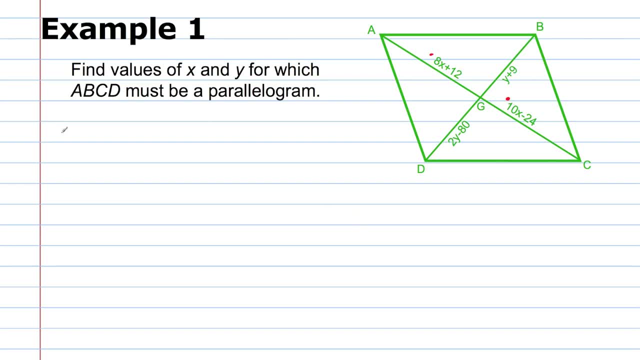 equal to 10x minus 24.. So we can write an equation from that 8x plus 12 is equal to 10x minus 24.. Now the other equation that we can write comes from the other diagonal: 2y minus 80 has to be equal to y plus 9, and the reason they have to be equal to each other. 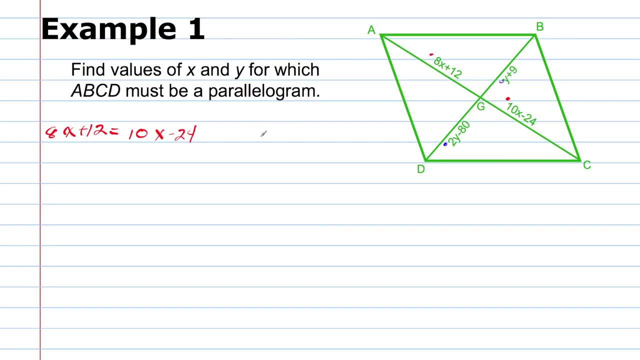 for this quadrilateral to be a parallelogram, the diagonals must bisect each other or have equal lengths. So the other equation is: 2y minus 80 is equal to y plus 9.. First I'll solve the equation, This equation. there's a couple ways to solve it. 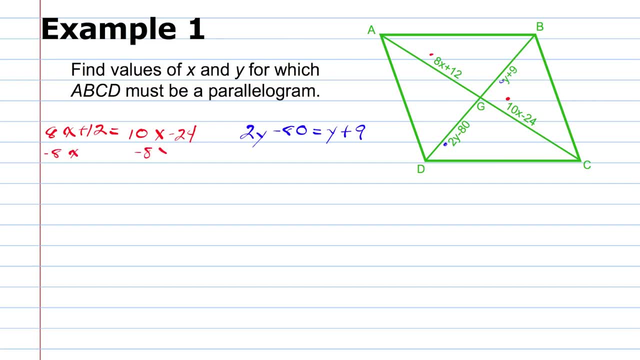 First, I'm going to do two things here. in the first step, I'm going to subtract 8x from both sides, which is going to get the x on the right of the equation, and at the same time I'm going to add 24, not 12.. 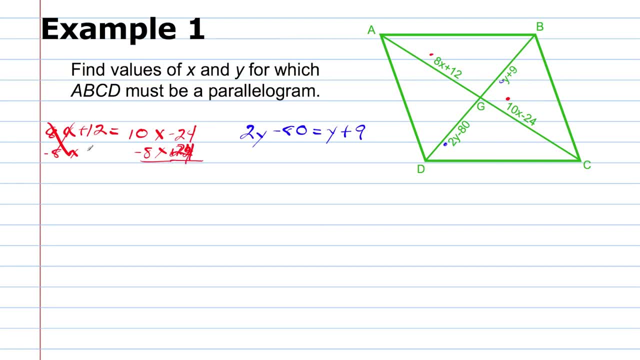 I just wrote 12 there, but that should have been a 24.. Adding 24 to both sides, 12 plus 24 is 36, on the right hand side, 10x. take away. 8x is 2x. 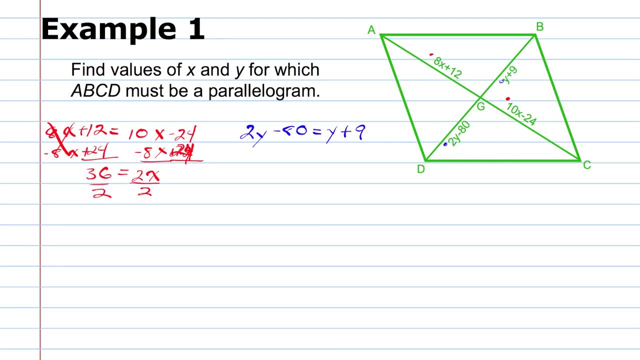 I next divide each side by 2.. The 2s on the right divide out, leaving x being equal to 36 divided by 2, which yields 18.. Therefore, the value of x- for this to be a parallelogram- is 18.. 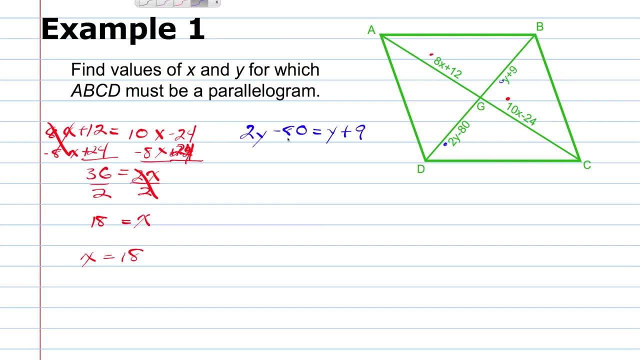 The other equation is a little bit easier to solve, not that the one in red was hard, but in this case I'll subtract y from both sides of the equal sign. That'll eliminate the y on the right hand side. So 2y take away, y is y. 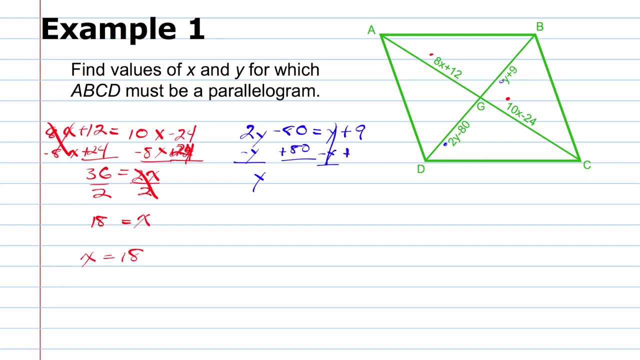 Then I will add 80 to both sides, which is going to give me, on the right hand side, 89. So the value of y- to make this a parallelogram- is 89.. So the two solutions here—x is equal to 18, and y is equal to 89.. 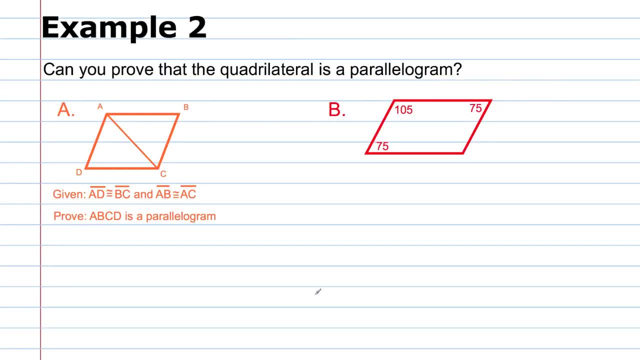 In example two we are adding our results here. Now we've got a piccznieرة. How many pic�i, How many picondoeng We're going to add? asked to determine if we can prove that a quadrilateral is a parallelogram. 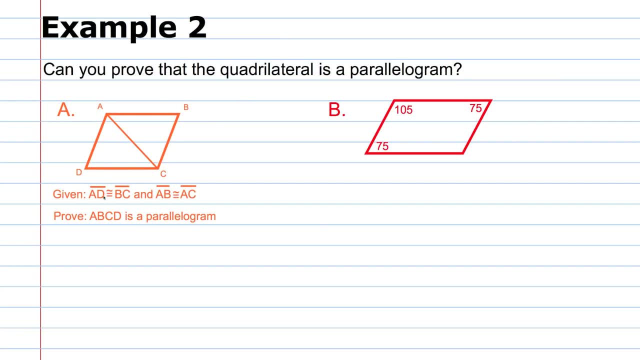 Here in the orange example, part A, we are given that segment AD is congruent to segment BC, so that's one pair of opposite sides congruent, and we are told that segment AB is congruent to segment AC. Can we prove that quadrilateral ABCD is a parallelogram? 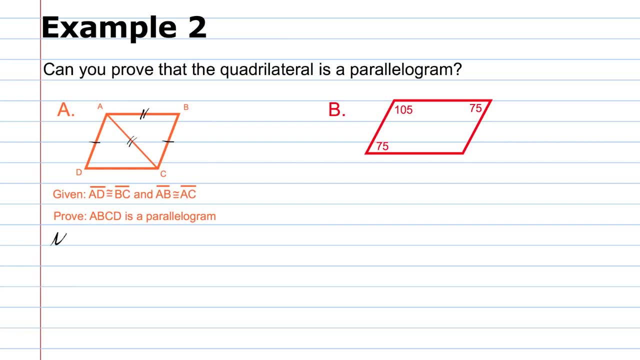 Well, with what's given here, we cannot prove that this is a parallelogram and for the given information, since it's talking about sides, we would have to have opposite sides congruent for this to be a parallelogram. So since we don't have all the information about opposite sides, we cannot determine. 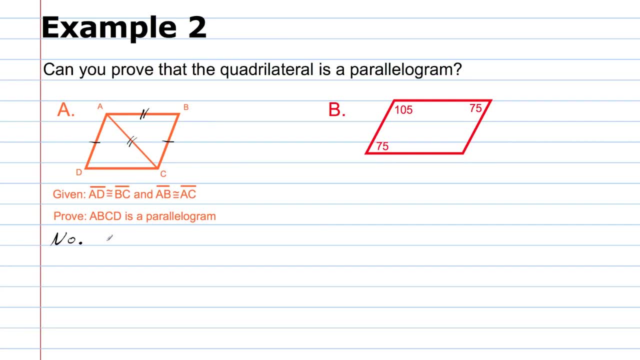 that this quadrilateral is a parallelogram, And another way to put that is that we do not know that AB is congruent to DC. If we knew that AB was congruent to DC, then opposite sides are congruent, which means this would be a parallelogram. 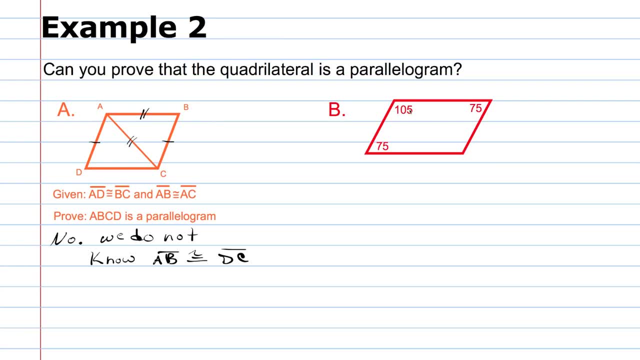 In example B, this red example. This is a parallelogram. This is a parallelogram. This is a parallelogram. For example, we're given the measures of three of the four angles of this quadrilateral by the polygon angle sum theorem. 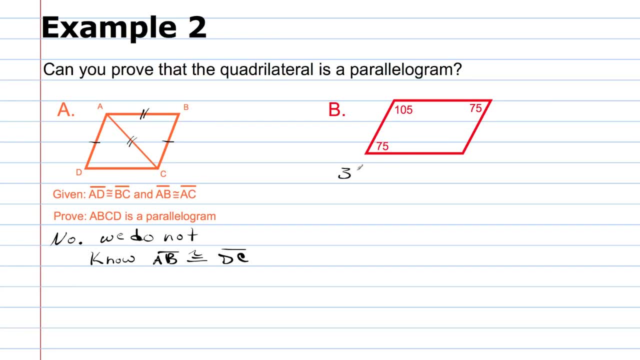 If we add all four of these up, it should be equal to 360.. Now we have one pair of opposite angles, congruent, so what we need to do, then, is find the measure of this missing angle, and I'm just going to label that x. 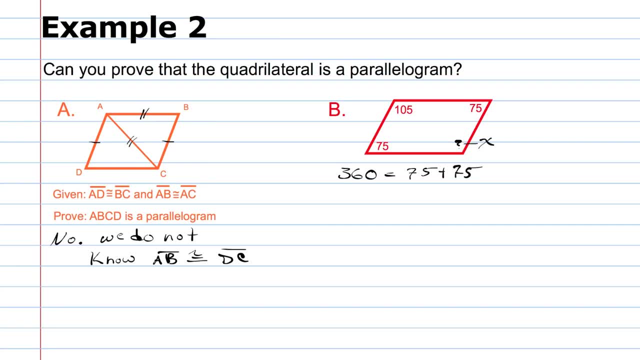 So we know that 75 plus 75 plus 105 plus x is equal to 360.. Solving this equation: when I add 75 and 75,, that gives 150.. And 150 plus 105 is 155.. It should be 255, not 155. 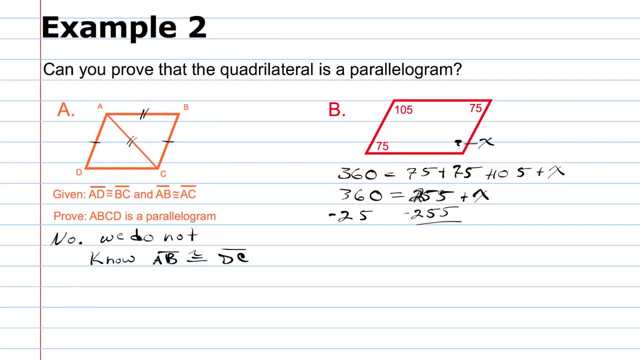 Then I subtract 255 from both sides, And one I complete, I get 255.. I add 75.. I add 75.. I add 150. And I complete, I add 75.. that subtraction, I end up with the missing measure as 105.. So, since I can show that opposite angles,